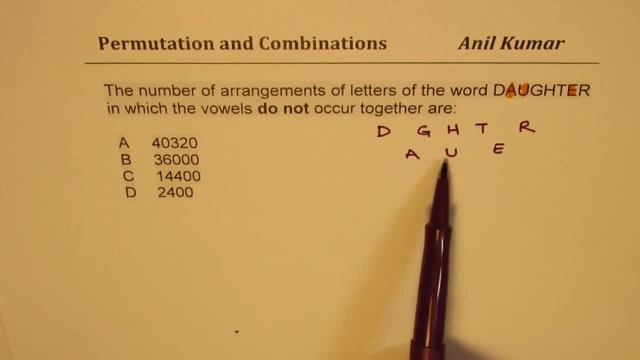 The question is that these vowels A, U, E should not be together. okay, That is the question. Now let me discuss with you how we end up getting wrong answers. Some of the students will say: well, there are 1,, 2,, 3,, 4,, 5,, 6,, 7, 8, and so the answer is 8, factorial, or which is 4-0, 3-2-0. 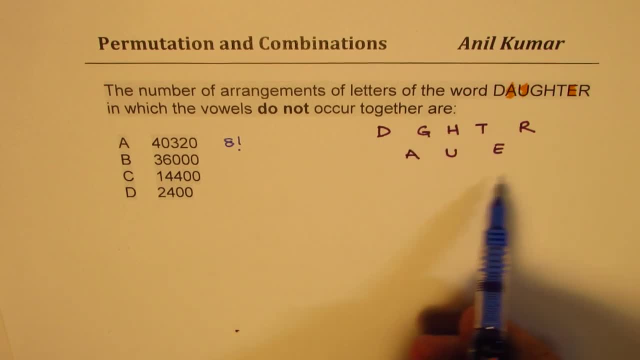 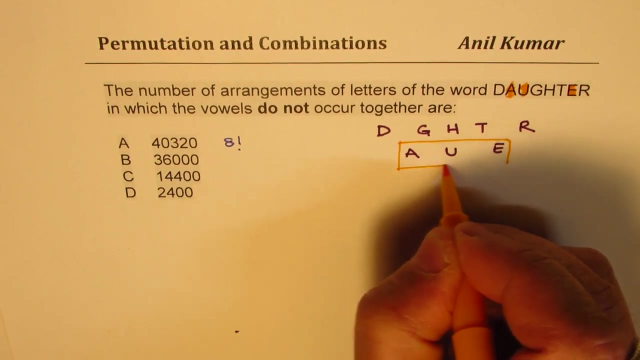 Well, definitely not. These are definitely the total number of ways in which you can arrange these eight letters. Some of us, what we do is that we kind of combine these three and then say, well, total is 8, factorial. but what we should do is that 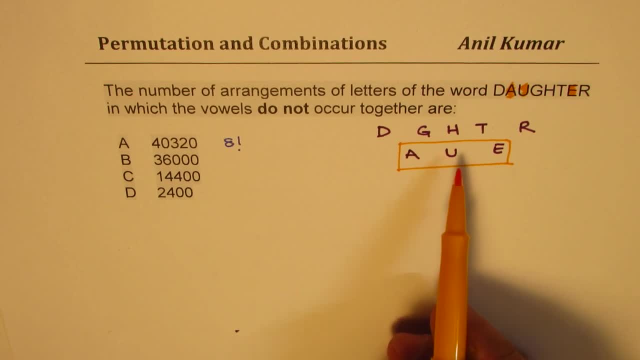 we should combine them all and find total number of ways and then subtract from 8 factorial Well, they say: well, now we have 1,, 2,, 3,, 4,, 5, and 1, there 6 factorial right. 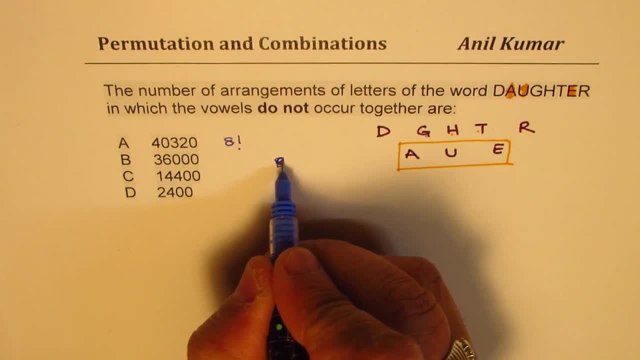 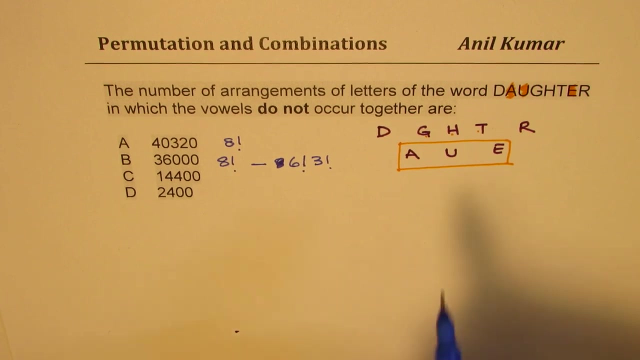 So we have this as 6 factorial. I mean, okay, 6 factorial times. these are three different letters, so times 3 factorial and we can take away from 8 factorial to get our answer. So that will ensure that all three of them are not together. 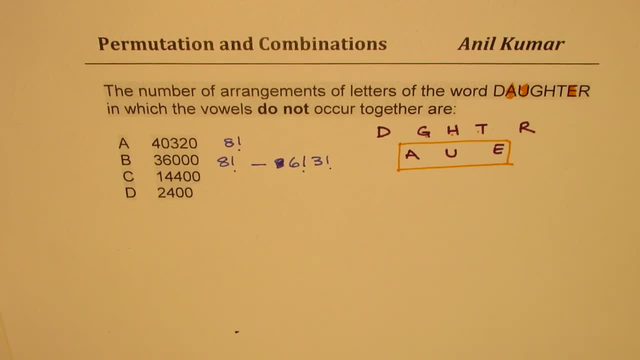 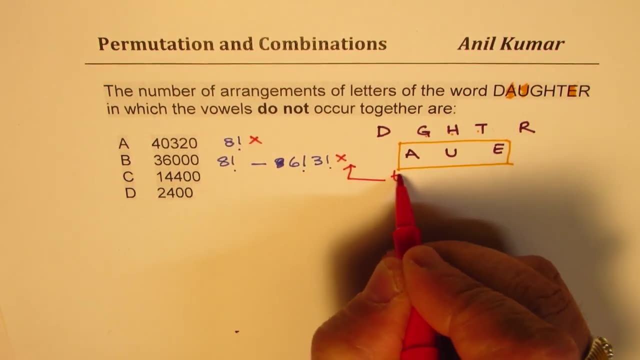 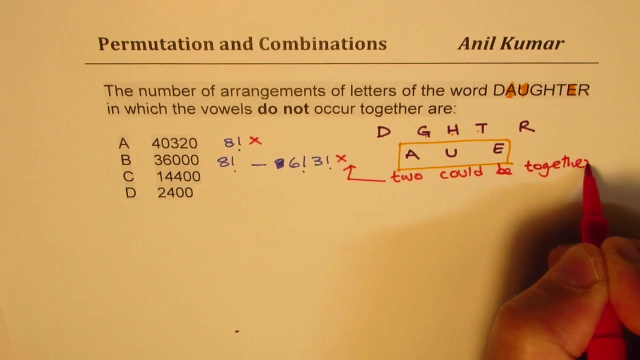 Well, two of them could be together. So this is wrong. and this is also wrong because in this case, two could be together. So what is the right solution? That is what we are going to look into now. right? So now let's look into correct solution. 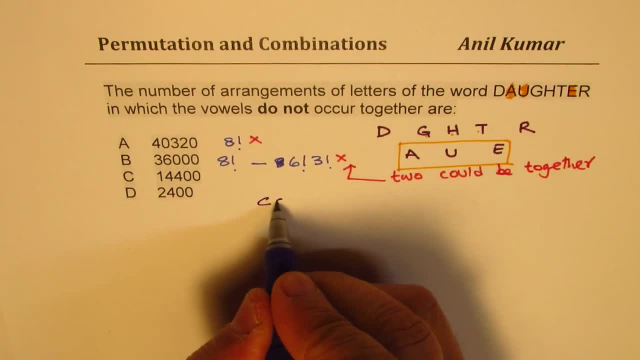 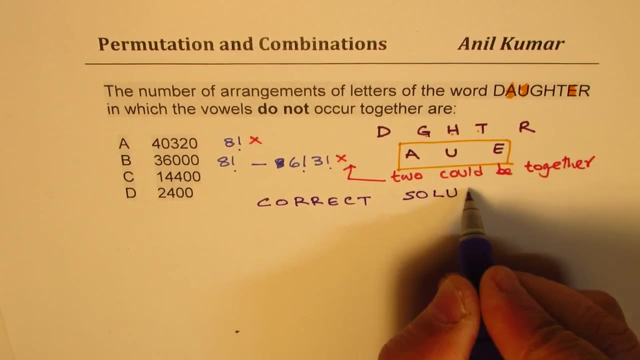 You can also pause the video, answer the question and then look into my suggestions. So now let's talk about the correct solution. So what we are given here is the word daughter, Which has D A, you know, is not a vowel, so we'll keep it separate. 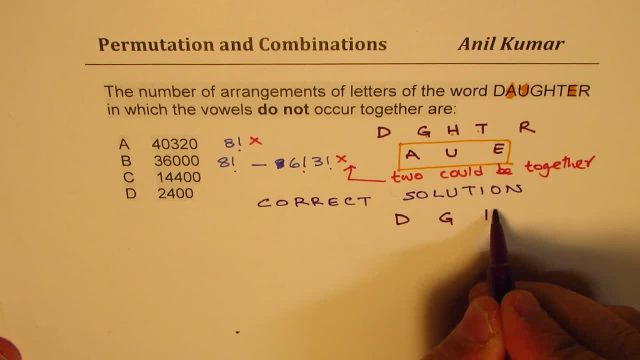 But we can have G, H, T and R- I mean sorry R- right Now. what we will do here is that we'll arrange the letters which are not vowels, which are 1,, 2,, 3,, 4.. 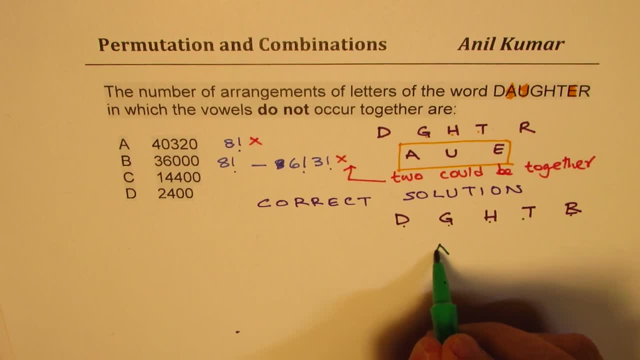 And 5, right, Three of them which are vowels, which are A, U and E, we can insert in between, ensuring that they're always separate. You get my idea. So that is how we actually find the solution. 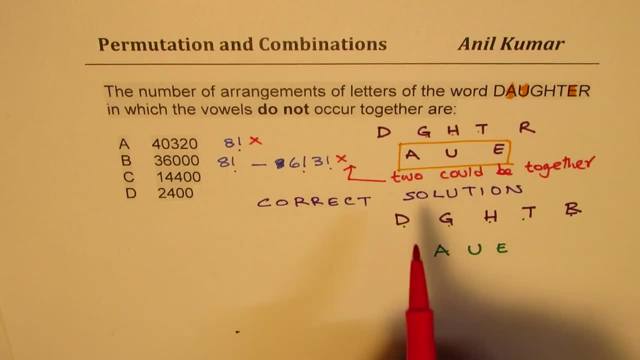 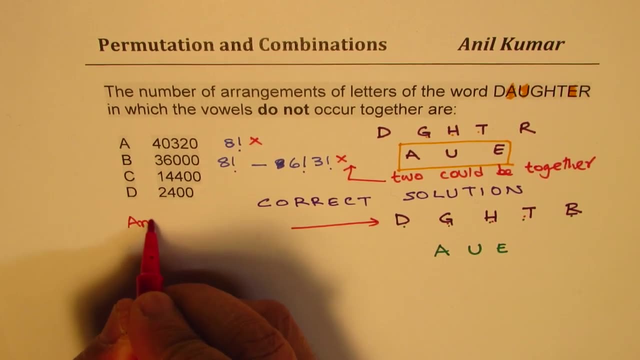 So the solution for this question is number of ways in which 1,, 2,, 3,, 4,, 5 letters can be arranged. So there are arrangements. So let's say, for example, A, U, E. 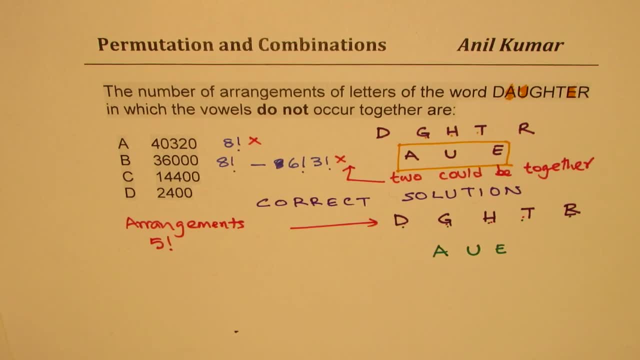 There are three different rooms. We'll have A, B, C and E And number of ways in which A U, E can be arranged, So we can have R, D, C and E. So this is the way. 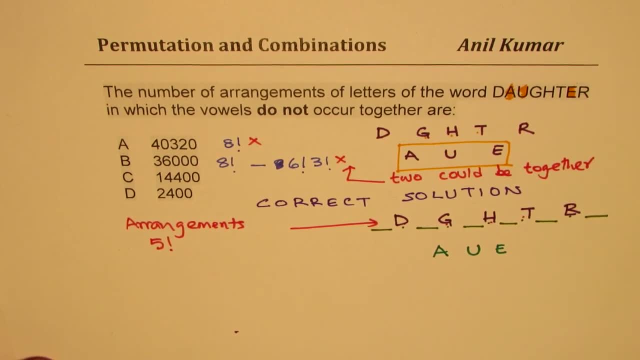 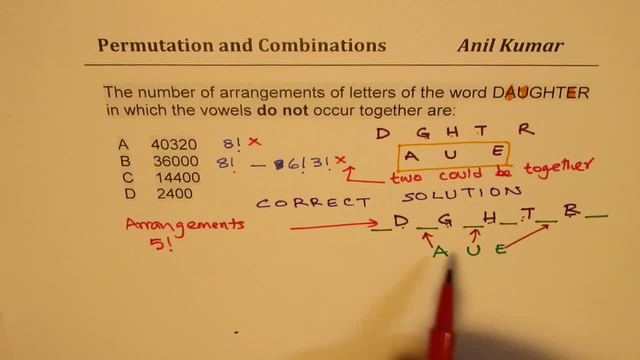 them will be together. You get an idea. Now. how many ways are there to insert three letters in one? So we have one, two, three, four, five, six in six spaces, So that is 6P3.. Therefore. 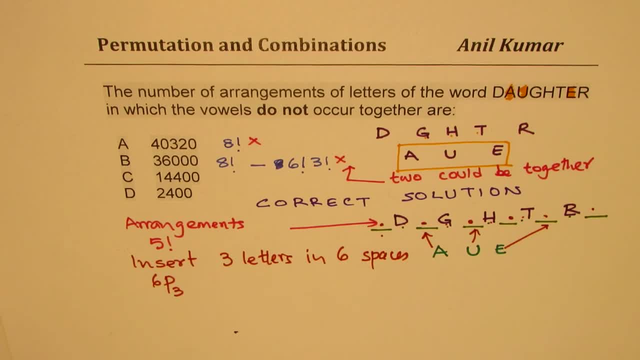 the total number should be how much? So the correct solution here is product of these two right. So in all these arrangements we could insert AUE in the spaces in between. So it is 5 factorial times 6P3.. That is the correct solution. So let's figure out how. 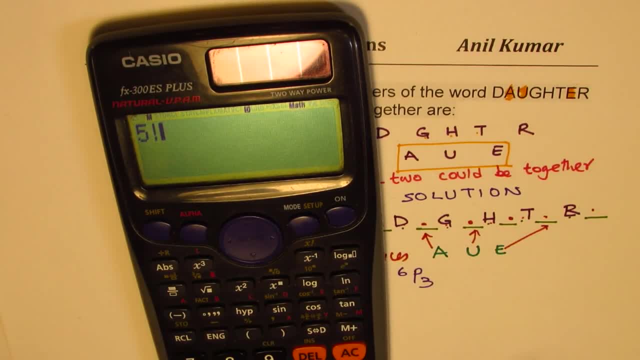 much it is. So we have 5 factorial times 6P3.. So that is the correct solution. So let's figure out how much it is: 6P3 and that is equal to 14400.. So these are the total number. 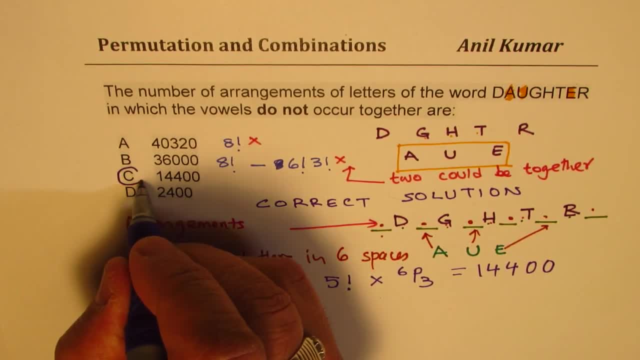 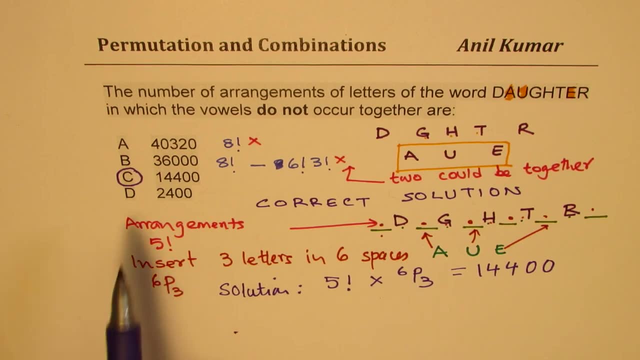 of ways, which is option C. Now, some of you could actually take 6C3.. So you'll get option D, which will again be wrong. You get my idea. So those are the three popular wrong answers for this question.